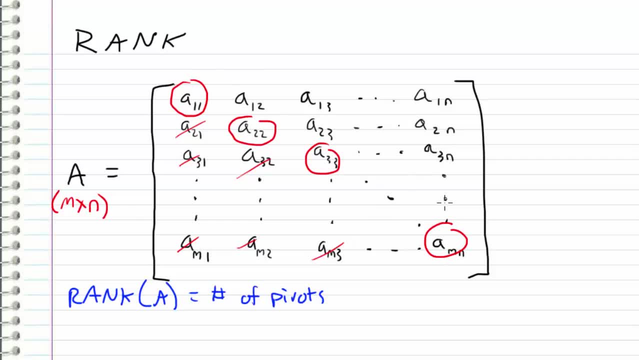 this until what we have is an upper triangular matrix where our pivots are the first non-zero entries in each row. So since each column in each row can have a maximum of one pivot, then we can also say that the rank of a matrix is equal to the number of 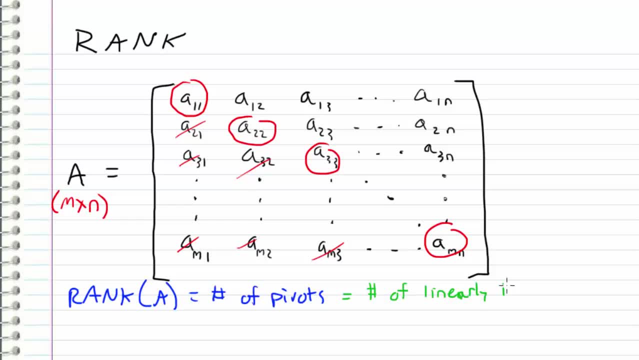 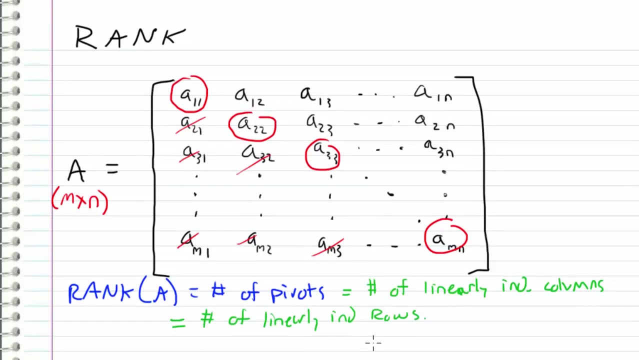 pivots in each row. So since each column in each row can have a maximum of one pivot, we can also say that the rank of a matrix is equal to the number of linearly independent columns and the number of linearly independent rows. But we have to recognize that the number of 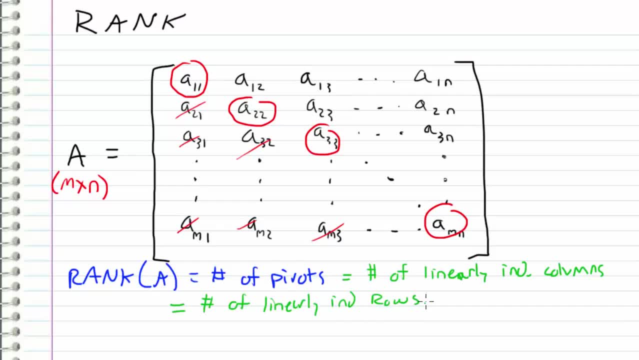 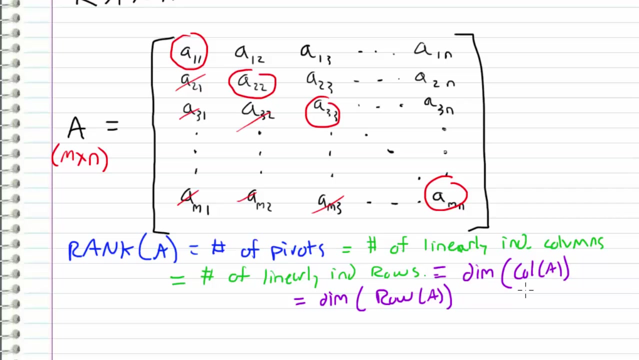 linearly independent columns and the number of linearly independent rows is the same thing as the dimension of the column space of A and the dimension of the row space of A, Or in other words, the rank of a matrix is equal to the number of basis vectors in the column space of A or the number of basis vectors in the row. 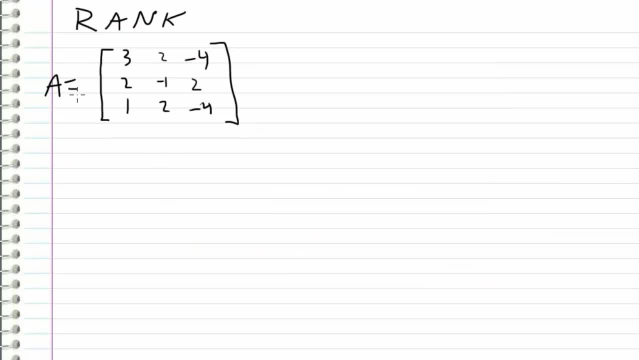 space of A. So let me demonstrate this concept with this example. If I have this matrix A, which is a 3x3 matrix, and I want to find the rank of this matrix, I can do so in multiple different ways. Otherwise, I can either find the number of pivots, 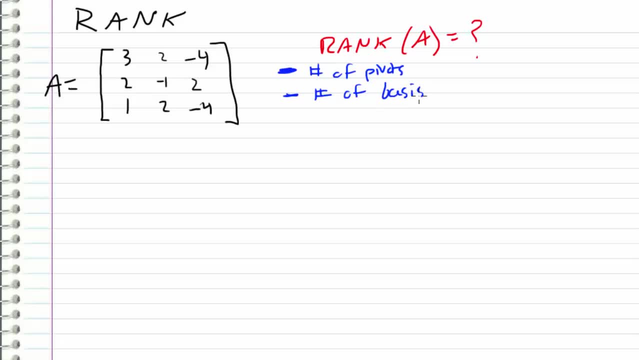 I can find the number of basis vectors in the column space of A, Or I can find the number of basis vectors in the row space of A, So let's go ahead and row reduce this matrix. So I have 3, 2, 1, 2,. 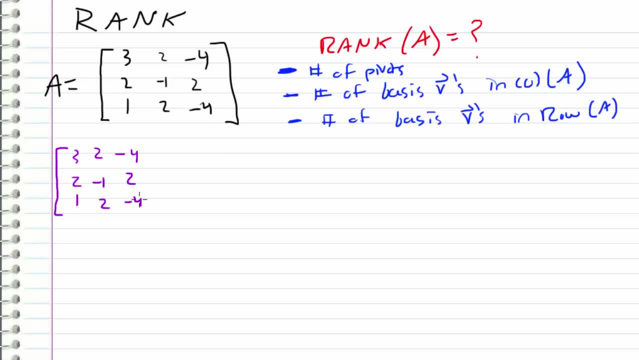 negative 1: 2, negative 4: 2, and negative 4.. So I'm going to start off with this pivot position and I'm going to eliminate everything below it. So I'm going to take the second row and I'm going to subtract 2 thirds times the first row And I'm going to take the. 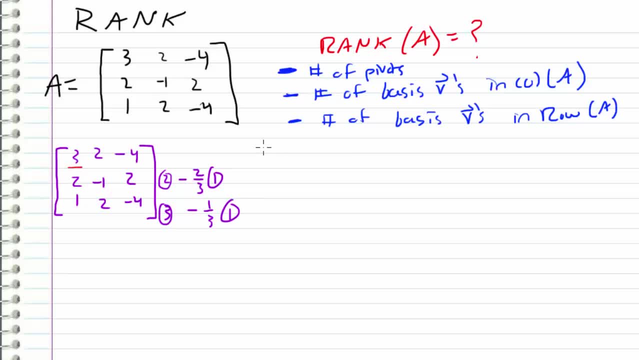 third row and subtract 1 third times the first row, And this gives us the matrix 3, 2, negative, 4, 0, negative, 7 thirds and 14 thirds, And in the bottom row I get 0.. 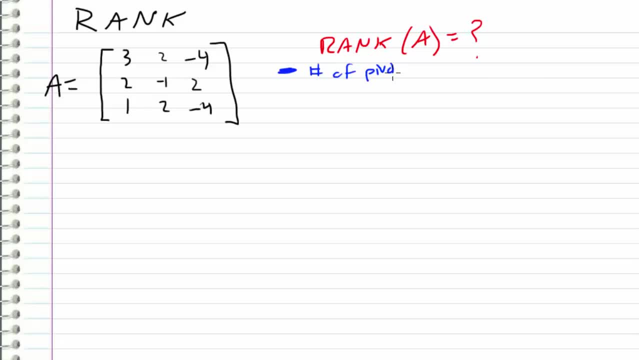 rank of this matrix. I can either find the number of pivots, I can find the number of basis vectors in the column space of A, or I can find the number of basis vectors in the row space of A. So let's go ahead and row reduce this matrix. So I have 3, 2,, 1, 2,. negative: 1, 2, negative 4, 2, 1, 2, negative 4, 2, 2, negative 4, 2, negative 4, 2, negative 4, 2,. 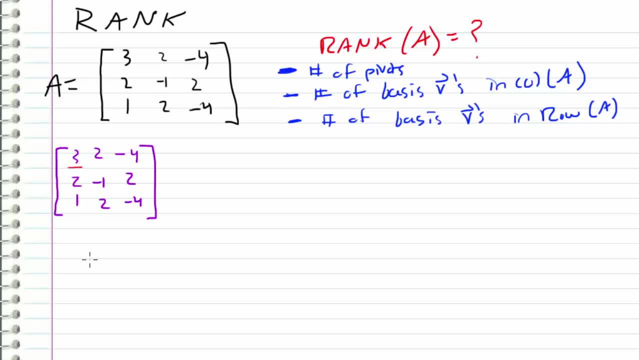 2, and negative 4.. So I'm going to start off with this pivot position and I'm going to eliminate everything below it. So I'm going to take the second row and I'm going to subtract 2 thirds times the first row, And I'm going to take the third row and subtract 1 third times the first. 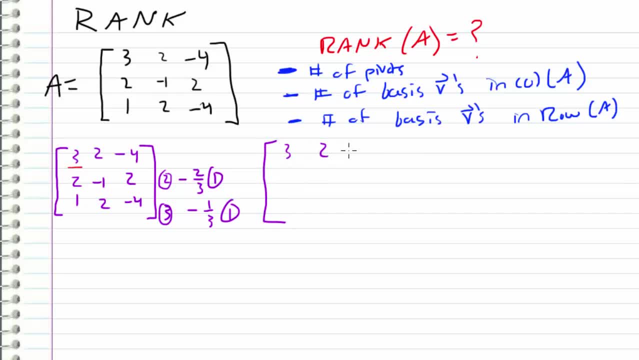 row And this gives us the matrix 3,, 2, negative, 4, 0, negative, 7 thirds and 14 thirds. And in the bottom row I get 0,, 2,, 1, 2, negative, 4, 0, negative, 7 thirds and 14 thirds. And in the bottom row I get 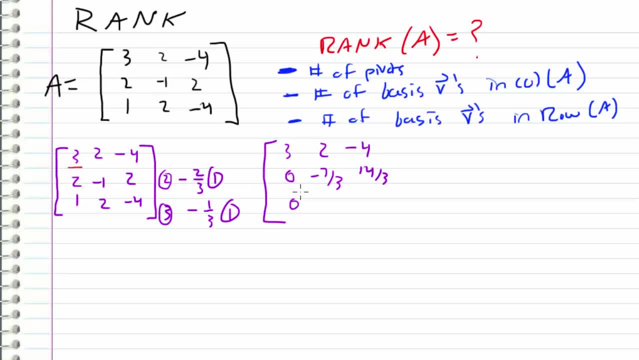 and then I have 6 thirds minus 2 thirds, which is 4 thirds. And then I have negative 12 thirds plus 4 thirds, which is negative 8 thirds. And now I'm going to move on to the next pivot position. 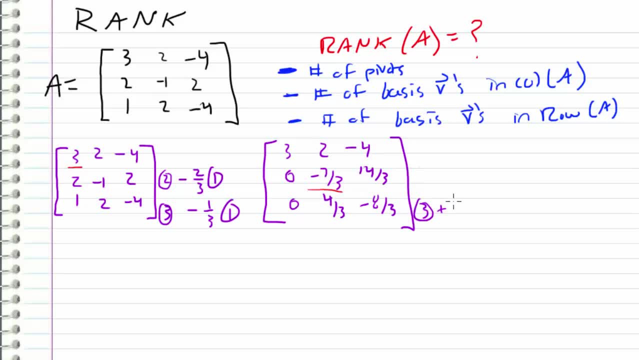 which is right here. So I'm going to take row 3, and I'm going to add 4 sevenths times row 2. And when I do this I get the matrix 3,, 2, negative 4, 0, negative 7, and 4.. 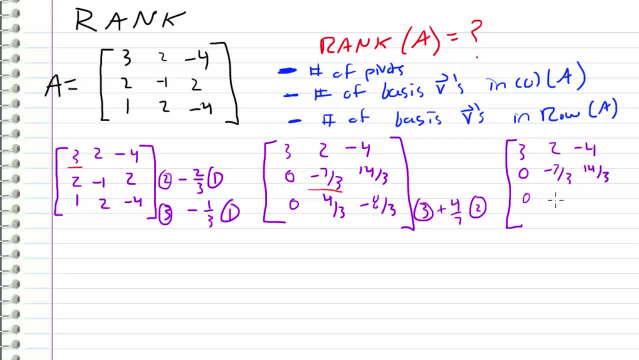 And then I have 7 thirds, 14 thirds- 0.. And then I have 4 thirds plus a negative 4 thirds, which is 0.. And then I have negative 8 thirds plus 8 thirds, which is also 0.. So this matrix is the row. 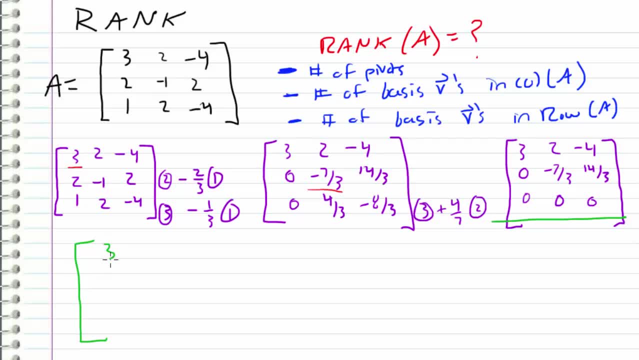 echelon form of A, And I'm going to rewrite this: 3, 2, negative, 4, 0, negative, 7 thirds, 14 thirds and 0, 0, 0.. So this is the matrix that we can use to find the rank of A. 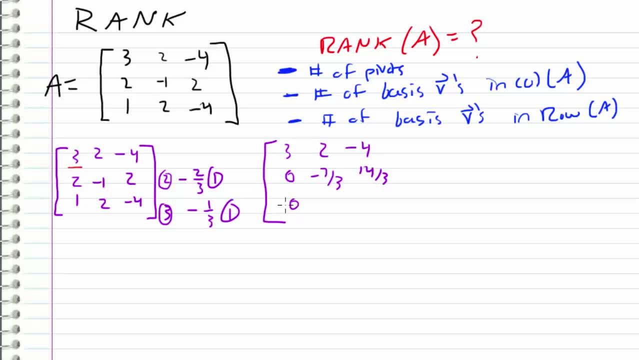 And then I have 6 thirds minus 2 thirds, which is 4 thirds. And then I have negative 12 thirds plus 4 thirds, which is negative 8 thirds. And now I'm going to move on to the next pivot position, which is right here. So I'm going to take 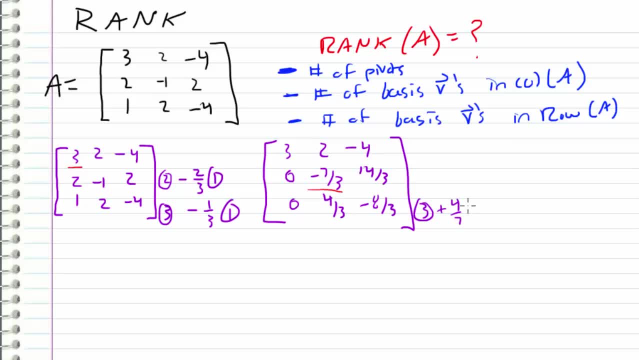 row 3.. And I'm going to add 4 sevenths times row 2. And when I do this I get the matrix 3, 2, negative 4, 0, negative 7 thirds, 14 thirds 0.. And then I have 4. 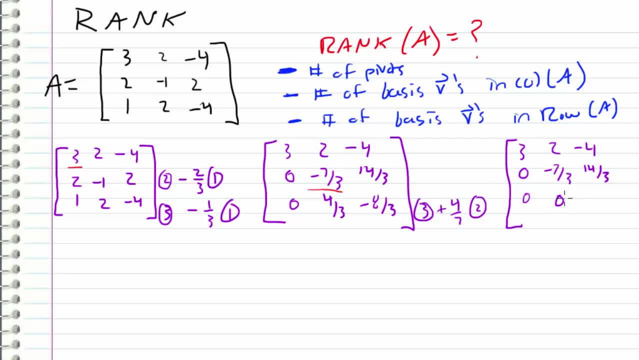 thirds plus a negative 4 thirds, which is 0.. And then I have negative 8 thirds plus 8 thirds, which is also 0.. So this matrix is the row echelon form of A, and I'm going to rewrite this. 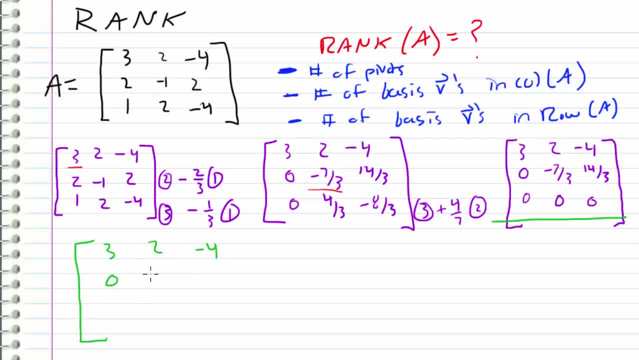 3, 2, negative 4, 0, negative, 7 thirds, 14 thirds and 0, 0, 0.. So this is the matrix that we can use to find the rank of A. The first thing that I want to point out is that these positions right here. 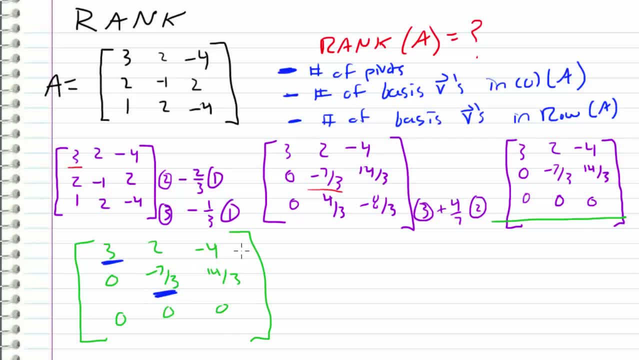 that I've underlined in blue are the pivot positions in this matrix, And these columns are the pivot columns. And then I could also circle the non-zero rows, which are these rows right here? So if you look at the basis for the row space, 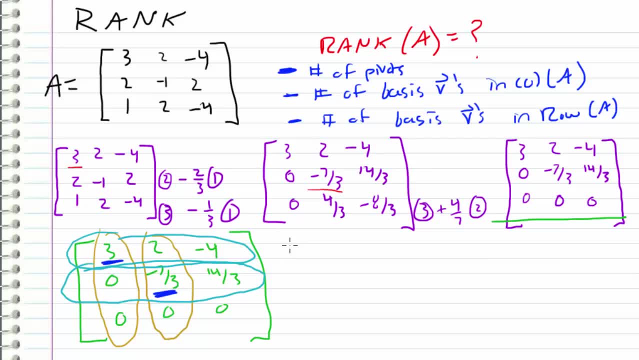 which are the vectors that I have circled in this light blue color. the row space of A is two-dimensional And that's because there are two basis vectors in the row space. If we look at the basis for the column space of A, we see that we have two basis vectors for the column space of A. 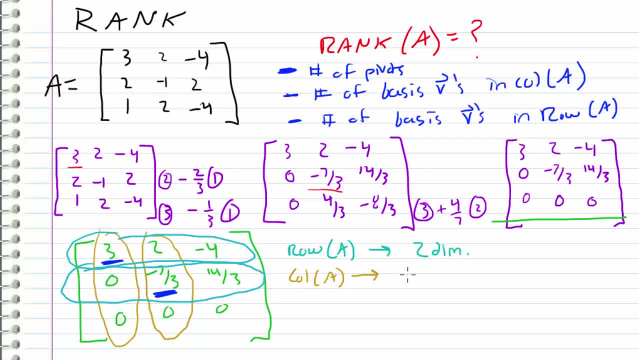 here. Therefore, the column space of A is also two-dimensional. And finally, if we look at the number of pivots, which I have in blue, then we can see that we have two pivots. So all this information means that we have a rank of our matrix equal to two. 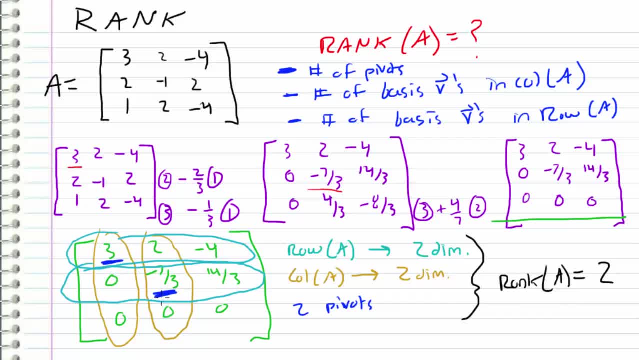 And the reason for this is because there are two pivots And, as a consequence of having two pivots, the row space is two-dimensional and the column space is two-dimensional because we select our basis vectors for the row space and column space from the rows and columns that contain the pivots.